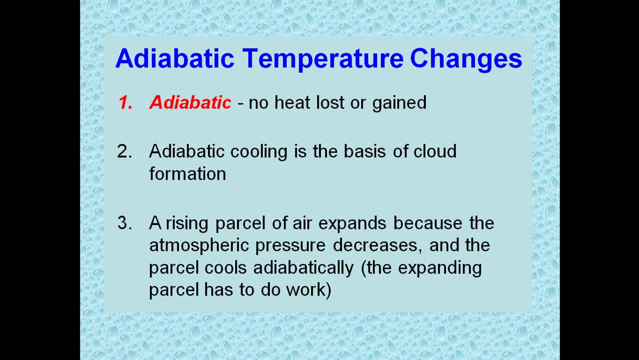 And so when an air parcel either rises or sinks, it either warms up or cools, And if we're talking about adiabatic changes in the atmosphere, that means that the air parcel is not giving off heat to the surrounding environment and it's not receiving heat from the surrounding environment. 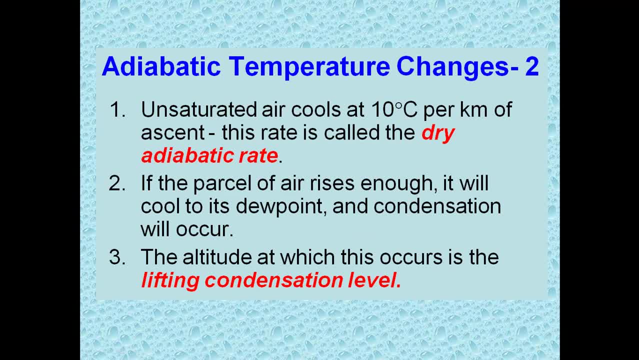 So that's what the term adiabatic means. So in the first week we talked about the environmental lapse rate or we talked about lapse rates in general. Remember that a lapse rate is simply just a rate of change of temperature with altitude. So 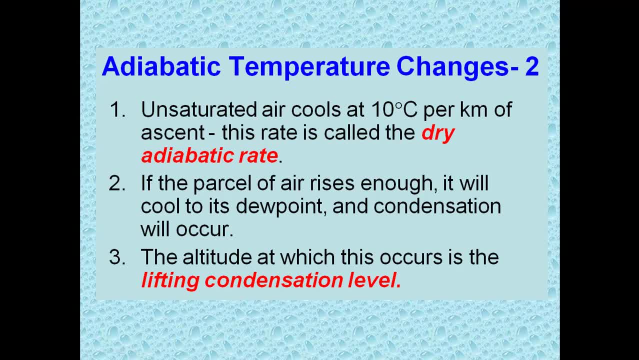 remember, as we travel higher in the troposphere, temperature decreases, But if we travel closer to the surface, temperature increases again. So that was the lapse rate definition, And we also defined what the environmental lapse rate was, which was the average lapse rate, And that was six and a half degrees Celsius per kilometer. 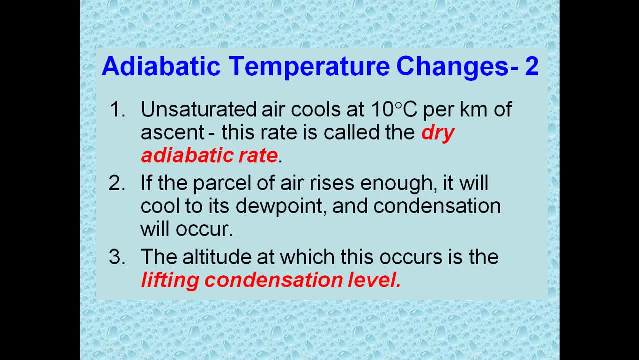 So that means temperature on average changes about six and a half degrees per kilometer as you change altitude. Well, I also mentioned in week one that lapse rates change all the time And even though we can take the average lapse rate, we can't use that all the time because meteorology is not a perfect. 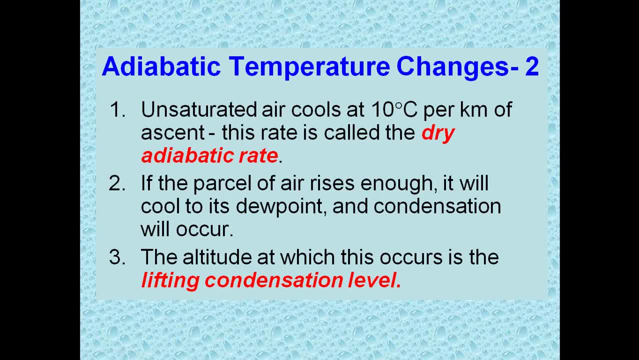 science. Therefore, our lapse rates aren't stationary, So I'm going to introduce two more terms to you. The first one would be the dry adiabatic lapse rate. This is the rate of change of temperature with altitude. when there is no more change in the temperature And we're going to use a 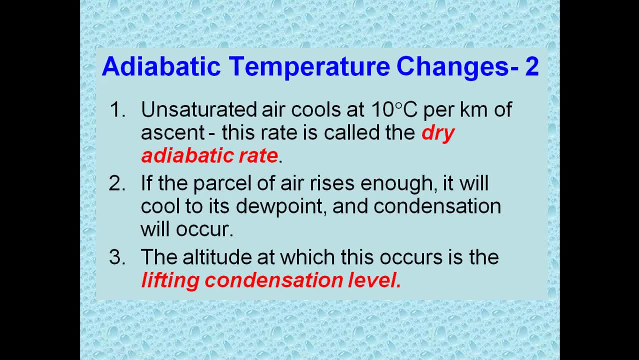 moisture present in the air parcel, or very little moisture in the air parcel. And so in the real world air parcels, if they're forced to rise, will cool at the dry adiabatic lapse rate. So they will cool at 10 degrees Celsius per kilometer until they get to a point in altitude where 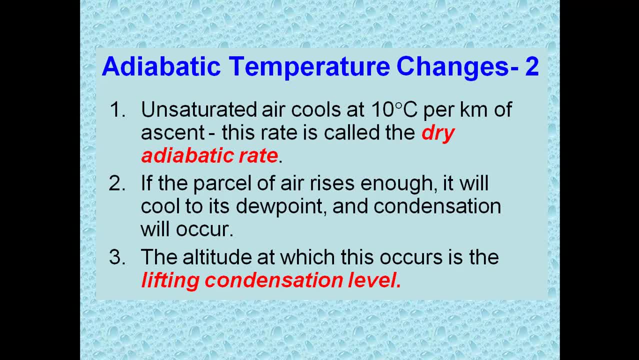 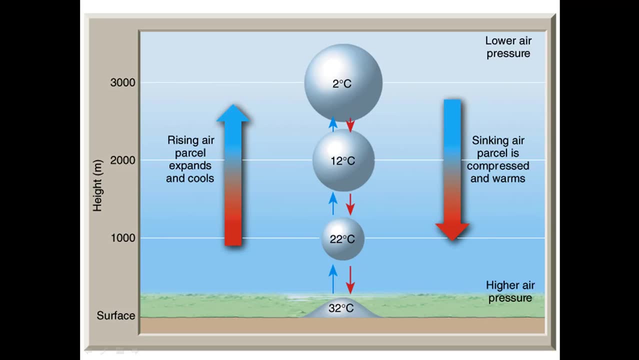 the air parcel has cooled off enough that it reaches its dew point, aka that the air parcel has already become saturated. At that level, clouds start to form, And this is what's known as the LCL, or the lifting condensation level. So, in a very basic representation, if you take an 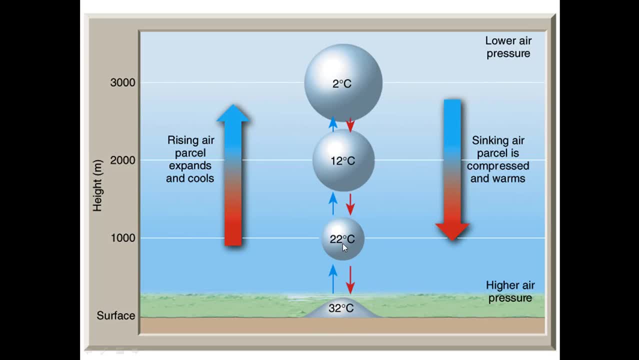 air parcel. that was 32 degrees at the surface. if you bring it to a height of one kilometer, which is the same thing as a thousand meters, you're going to have a very high condensation level. So if it rises another kilometer it cools off another 10 degrees. So here it went, from 22. 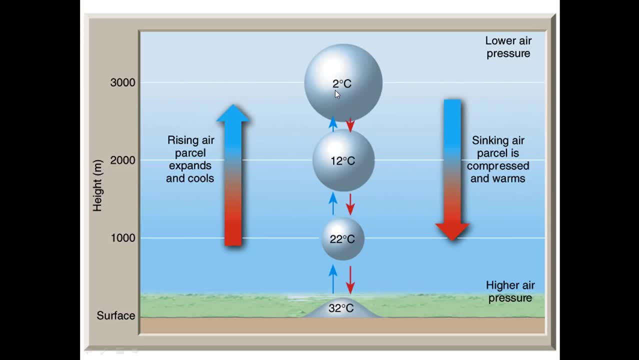 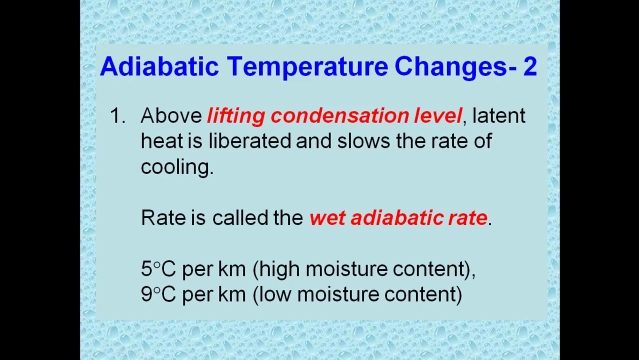 to 12.. And if it rises another kilometer, you can see here that the air parcel is now at two degrees Celsius, So it is cooled off once more. So that is what the dry adiabatic lapse rate is. It's just a rate of change. So above the lifting condensation level, 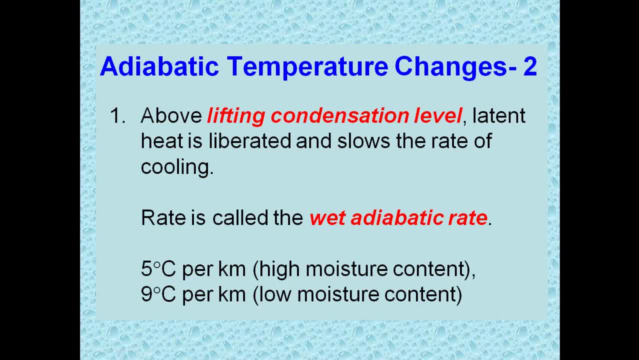 air parcels still continue to rise, but they rise at a slower rate, And that slower rate is what's called the wet adiabatic lapse rate or the moist adiabatic lapse rate, However you want to call it, it's the exact same thing. And when we talk about the wet adiabatic lapse rate, 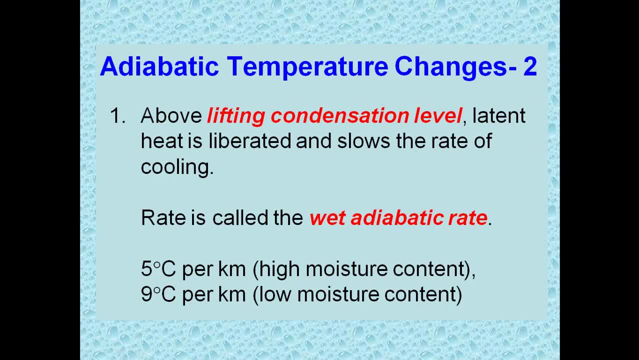 that is half of the dry adiabatic lapse rate. So air parcels will keep rising at a rate of five degrees Celsius per kilometer instead of the dry adiabatic lapse rate, which is 10 degrees Celsius per kilometer. So air parcels will continue to rise, but they'll rise at a slower rate. And 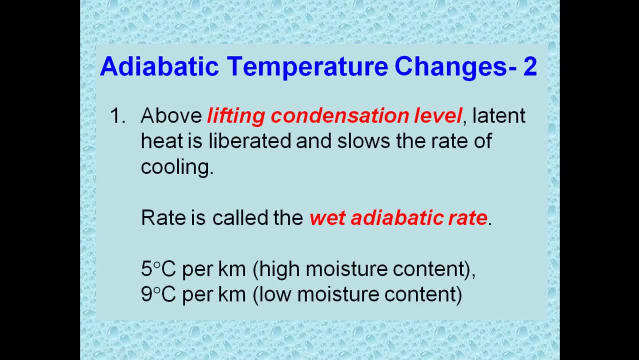 why is that? Well, once an air parcel has reached the lifting condensation level, that means that clouds are now starting to form. So now we're taking water vapor and we're condensing into water droplets, So we're going from a gas to a liquid, because that is what a cloud is. If you 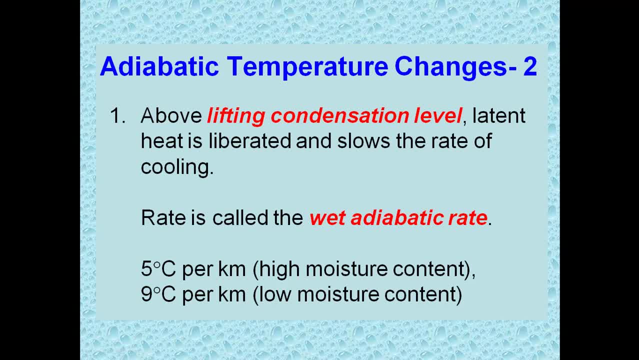 have ever been skydiving in your life before, it's the exact same situation. So if you have ever been skydiving in your life before, it's the exact same sensation as if you went to Six Flags or some amusement park where there was a long line in order to keep the crowds cool. They basically. 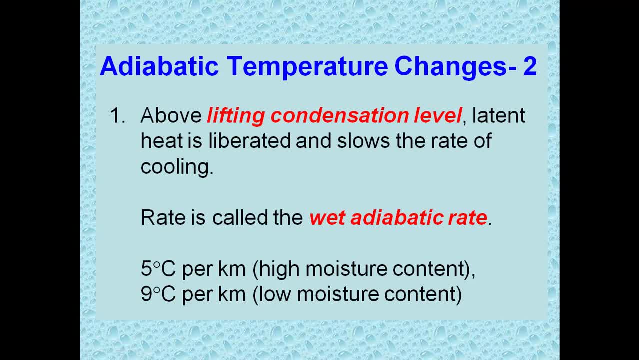 just had these mist tents to keep guests cool while they waited in line. That is essentially what a cloud feels like, And that's what a cloud is. It's just comprised of a bunch of water droplets, But at that point that is the liquid form of water. So remember what I said about. latent heat at the beginning of this video. If you have ever been skydiving in your life before, that is exactly what a cloud is. If you have ever been skydiving in your life before, that is exactly what a cloud is. If you have ever been skydiving in your life before, that is exactly what a cloud is. 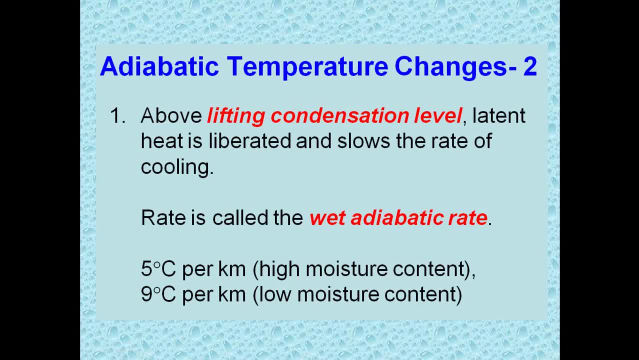 When you take gas or water vapor in this scenario, and you bring it back to liquid water, you have to cool the overall temperature of water. And when you cool the overall temperature of water, just like you would want to cool your body temperature, what would you do? You would want. 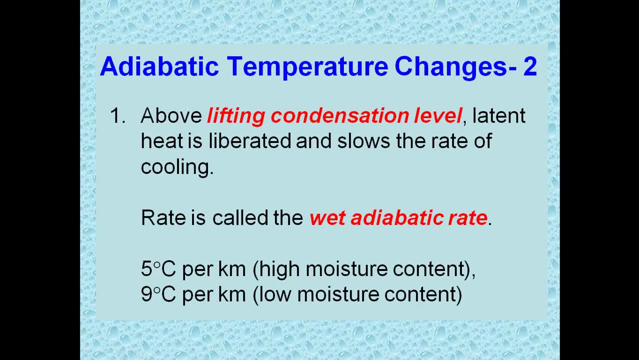 to release things that would keep you warm. You want to release heat. That is how humans physically cool down and that's how water physically cools down. It has to release latent heat. So that's why the wet adiabatic lapse rate is half of the dry adiabatic lapse rate. 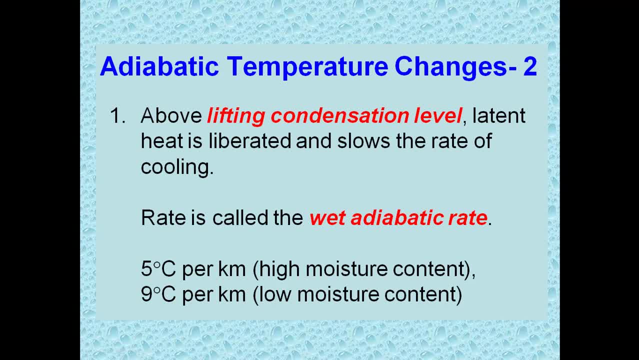 because, above the lifting condensation level, we're already building a cloud. Cloud formation has already happened. Therefore, we're changing water's state from a gas back to a liquid and therefore heat rises, but we have released latent heat and therefore we don't have. 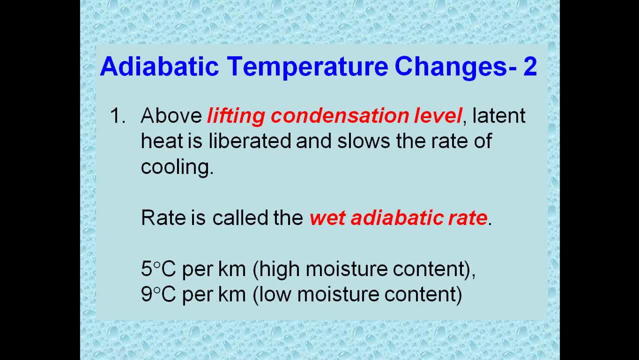 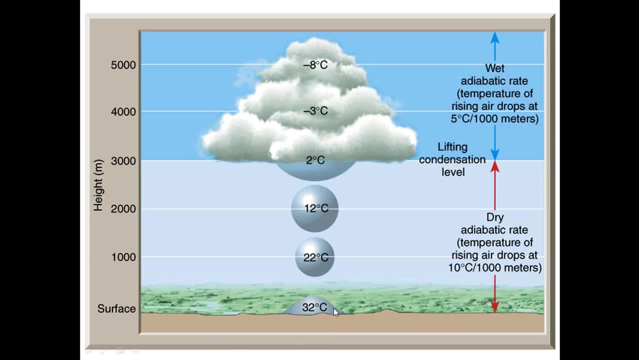 as much latent heat to play with, And that is why air parcels still rise, but at a much slower rate. So here you can see, we have the same air parcel. It's 32 degrees at the surface. We bring it up another 1 kilometer. It is cooled by 10 degrees Celsius. We bring 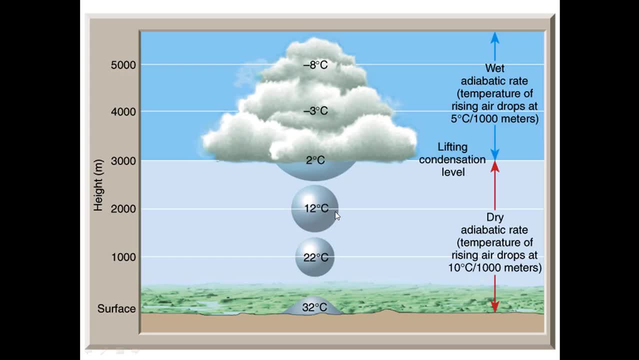 it up another kilometer, It is cooled by another 10 degrees, down to 12 degrees Celsius. But here, at 3 kilometers or 3,000 kilometers, it's cooled by another 10 degrees. So that's 8,000 meters. You see that this air parcel has now cooled to 2 degrees Celsius and has now 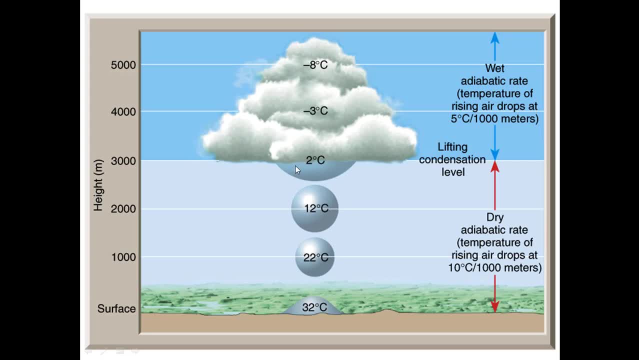 started forming a cloud. Well, that means at this level, 2 degrees was the dew point temperature in this air parcel. That means that we cooled this air parcel to the dew point and now our air parcels has become saturated. So here we start building a cloud, And so for every kilometer that 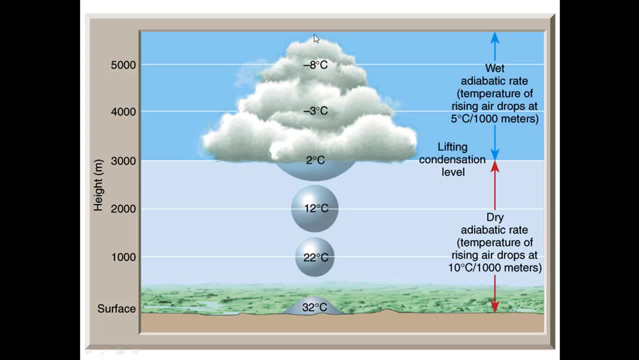 we travel. after that, the temperature still decreases because we're still traveling higher in the troposphere, but it decreases at a slower rate of 5 degrees Celsius per kilometer. So here is 2 degrees Celsius. We went up another kilometer and we just simply subtract 5 from this number.